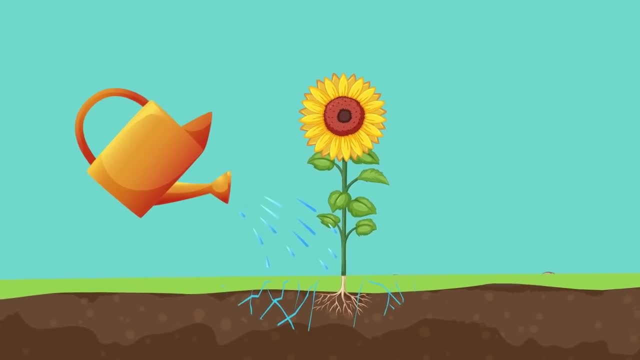 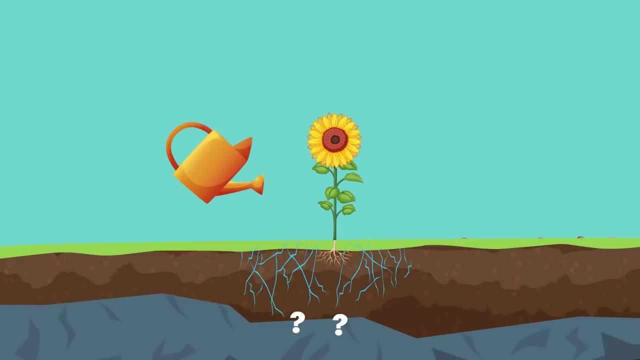 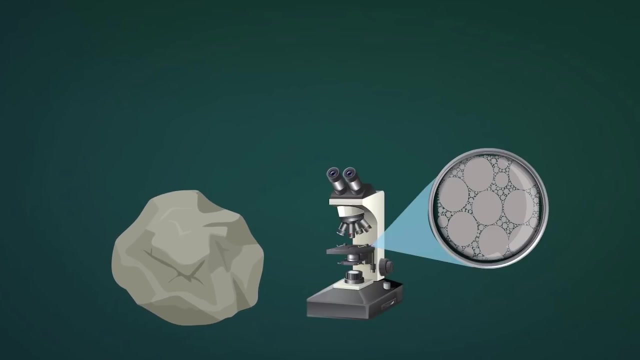 observe the water disappearing in the ground. But what happens when the water infiltrating downwards reaches the rocks that are under the topsoil? Well, it depends on what type of rock it finds. There are rocks that contain a lot of small holes, even though they are sometimes so small. 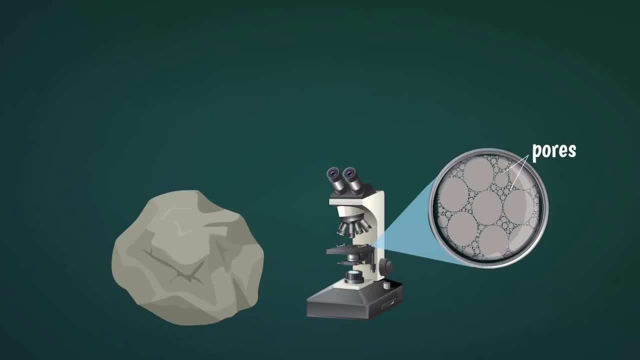 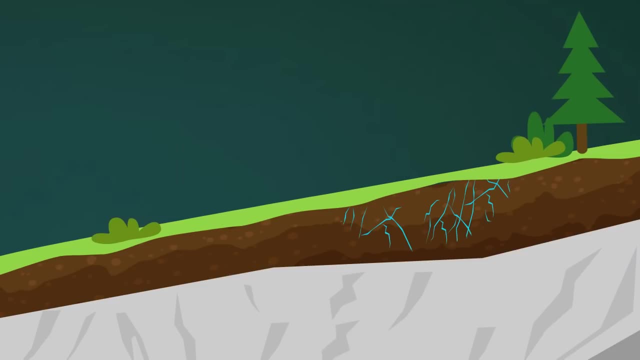 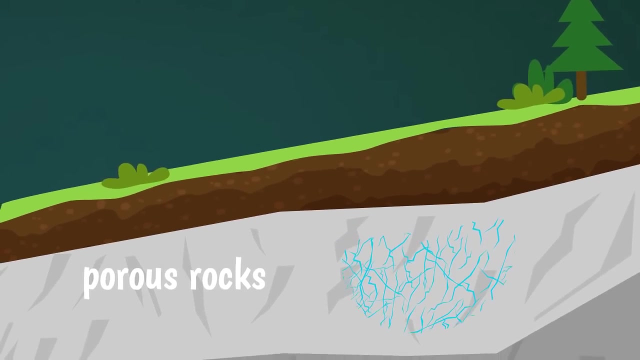 that you need a microscope to see them. These little holes are called pores, And rocks that have many pores are said to be porous. In general, when the rocks are porous, water can seep through the holes and continue its journey downwards, But there are also rocks that have very few pores. 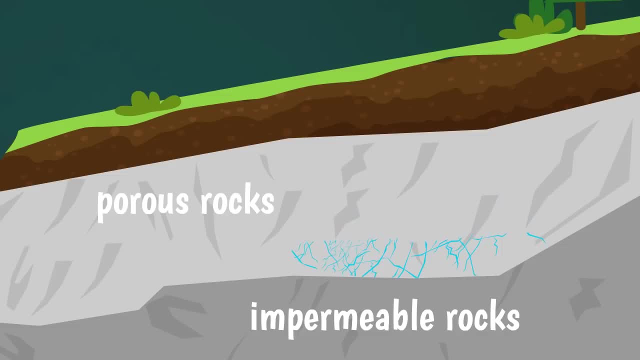 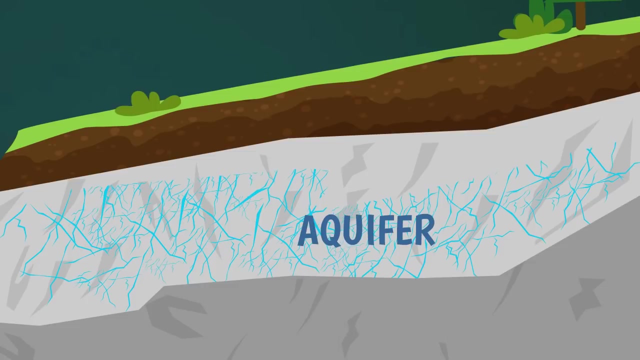 In this case, the rocks are said to be impermeable because water cannot pass through them. Now, if the downwards passage of water is blocked by a layer of impermeable rock, then water begins to collect in the porous rocks above. This way, it can form large underground reservoirs of water, known as groundwater aquifers. 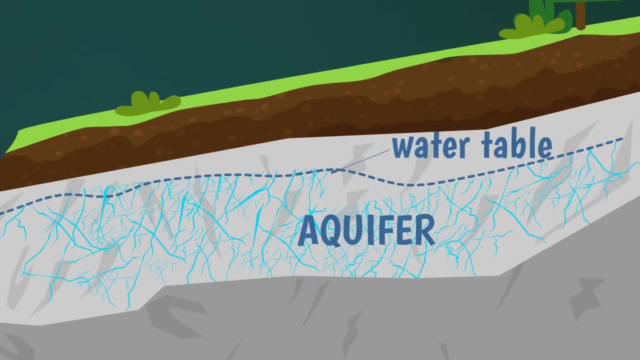 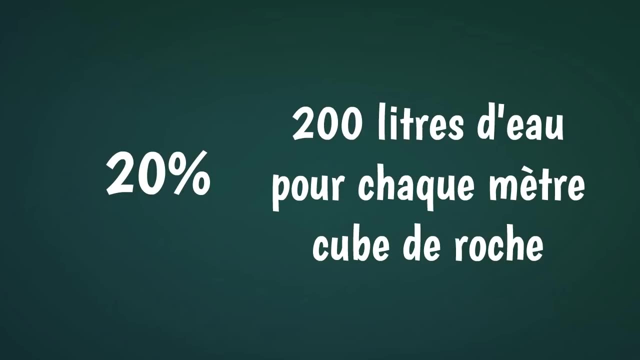 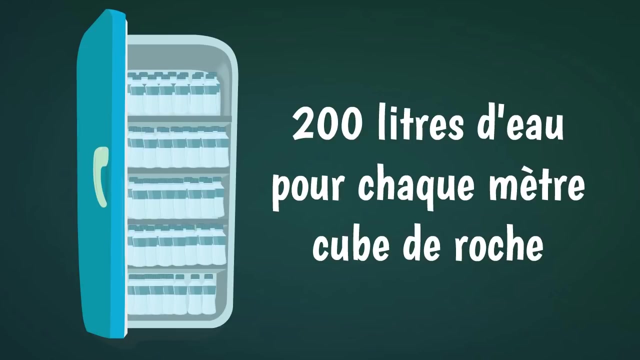 The uppermost level in which the pores contain water is called the water table. Rocks between the water table and the base of the aquifer can contain more than 20% of their volume of water, Which means that more than 200 liters of water per day can contain more than 20% of the water. 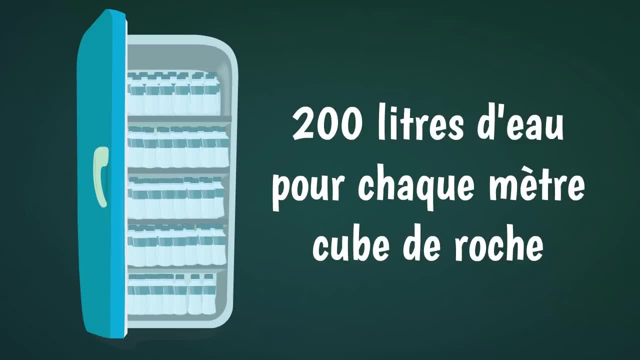 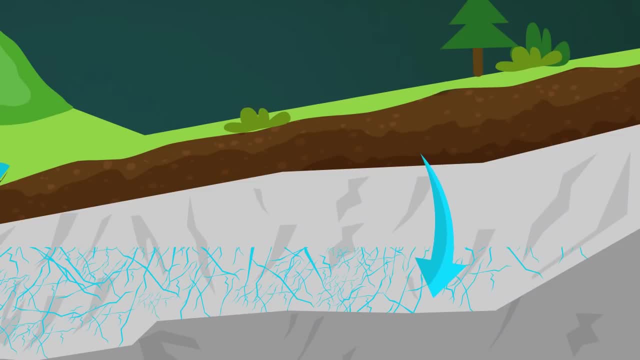 This means that more than 200 liters of water per day can contain more than 20% of the water. The water can be stored in each cubic meter of rock. A cubic meter is more or less the size of a fridge. When it reaches an impermeable layer, the water can no longer continue to infiltrate. 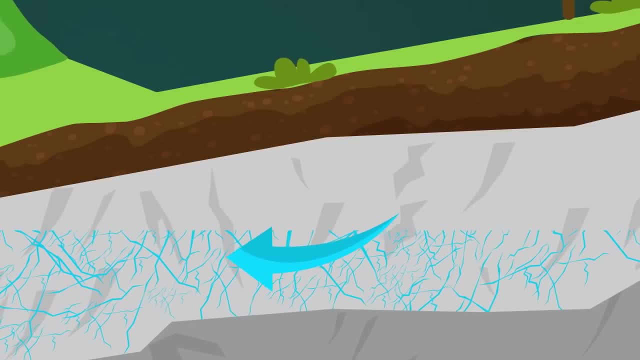 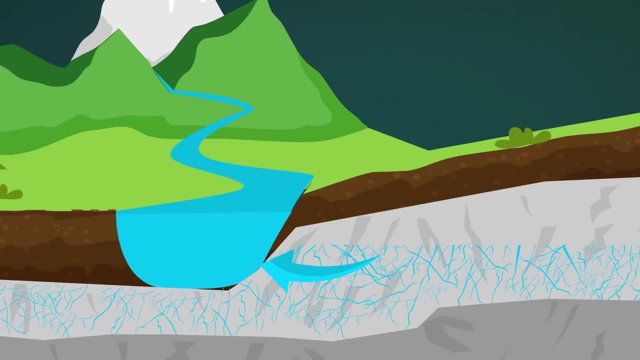 downwards. So it slowly moves, more or less following topography, towards places where the water table is the lowest. In some places, the water table might come all the way to the surface. In this case, the water can come out from underground and return to the surface. 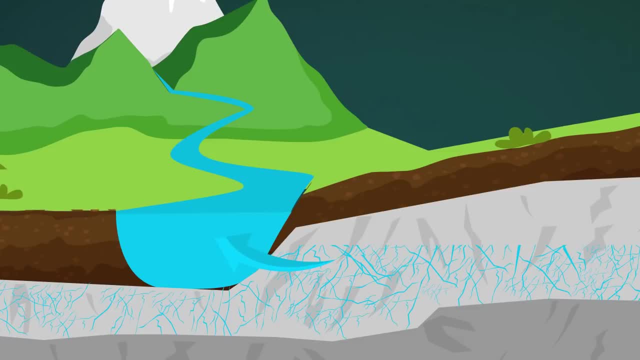 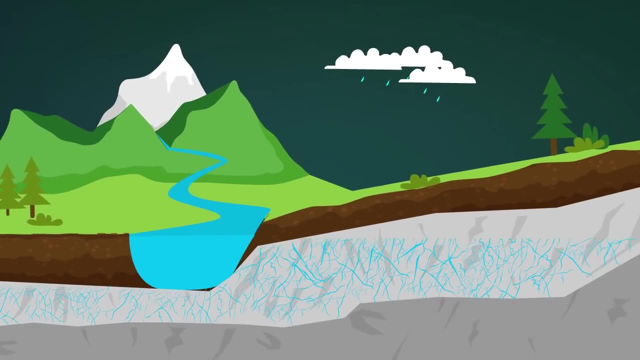 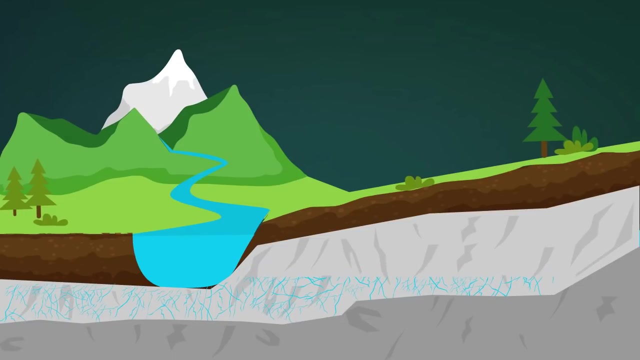 In fact, it is in this way that the rivers receive a lot of their water. The level of the water table rises and falls with the rain and the seasons, But as long as the level does not drop lower than the bed of the river, water will seep.